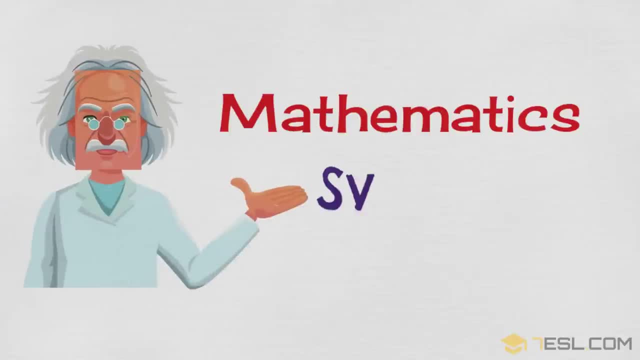 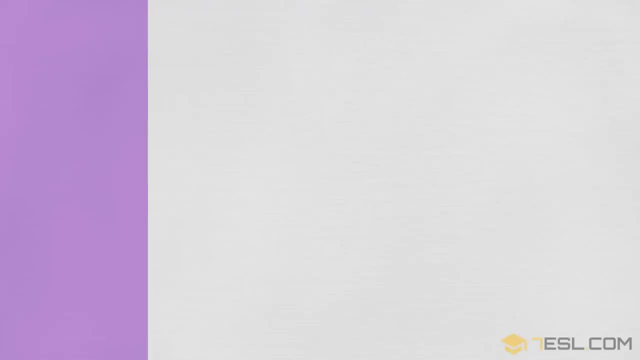 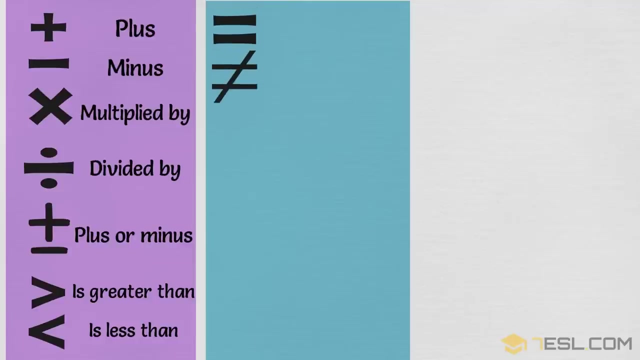 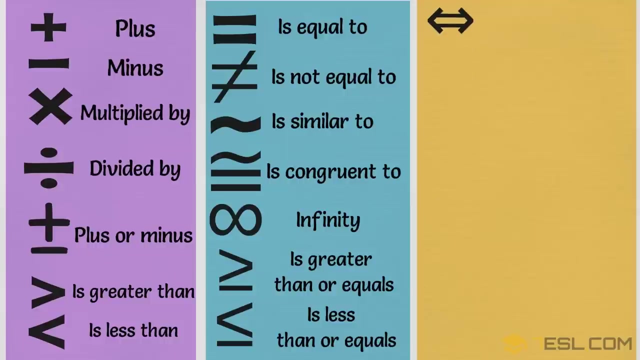 Mathematics Symbols: Plus- Minus. Multiplied by, Divided by Plus or minus, Is greater than, Is less than, Is equal to, Is not equal to, Is similar to, Is congruent to Infinity, Is greater than or equals, Is less than or equals Is equivalent to Implies Theta. 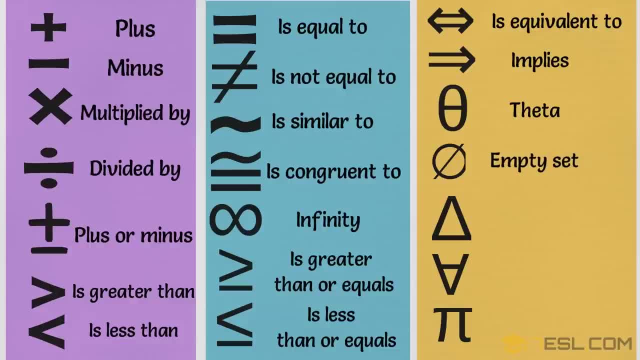 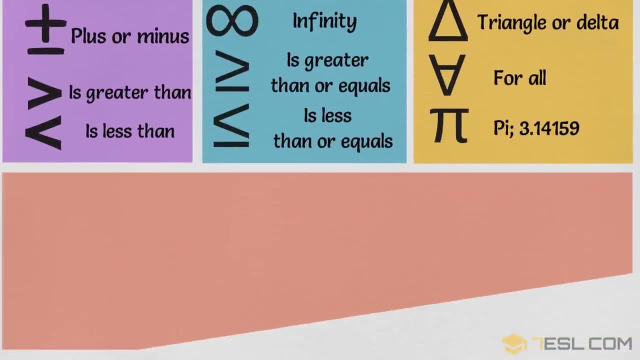 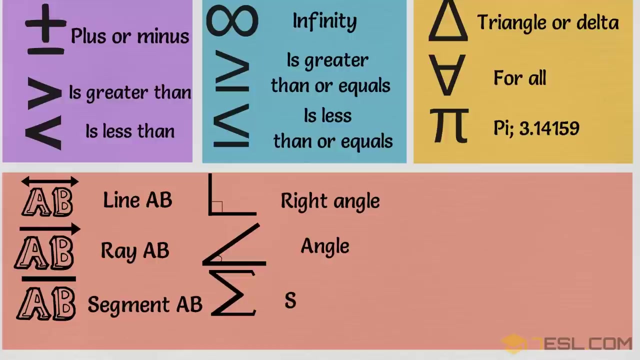 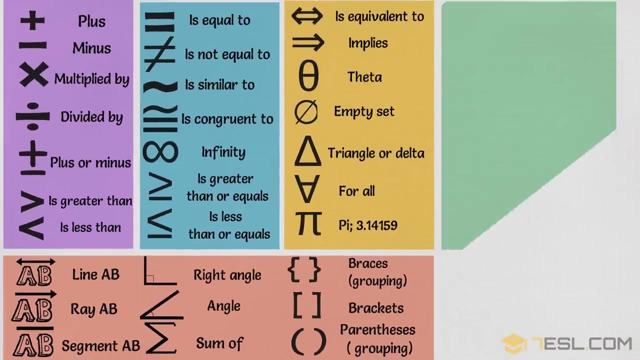 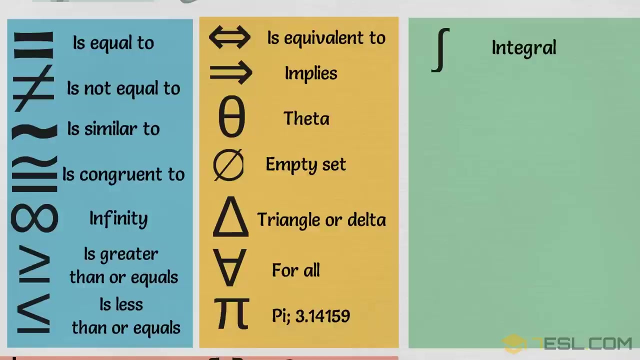 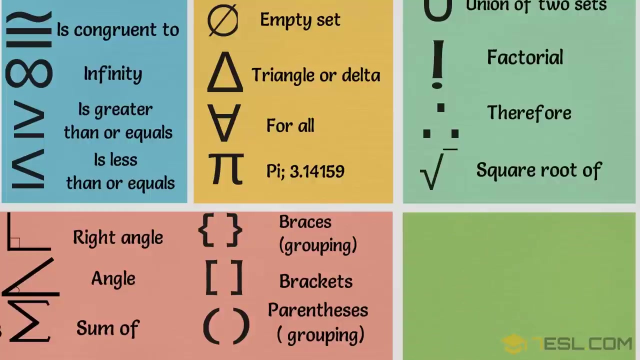 Empty set Triangle or delta For all. Pi 3.14159, Sub pus Limit, Complex Limit, Win Input Input. Input Input Tube, Intertrack, Angle, Sum of Braces, Brackets, Grouping, Integral Intersection of two sets, Union of two sets. Factorial, Therefore, Square root of Perpendicular. 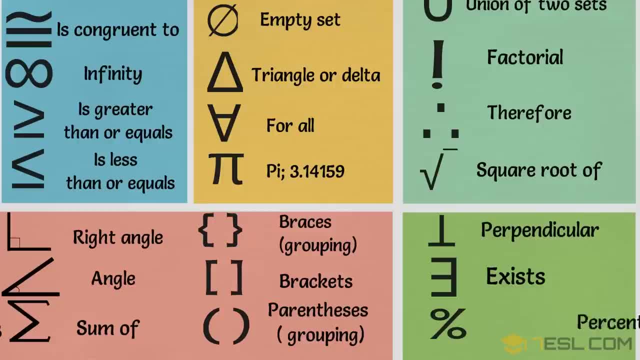 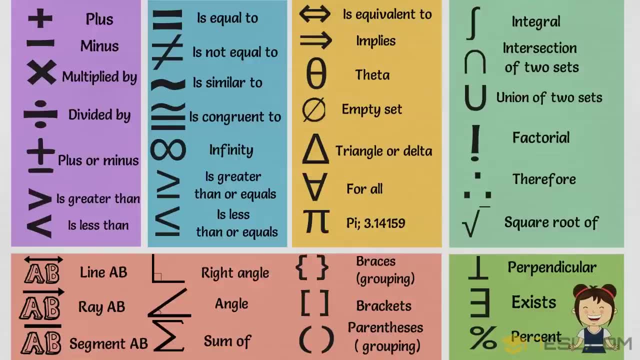 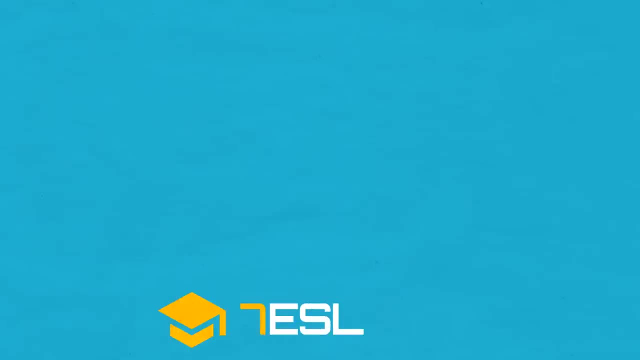 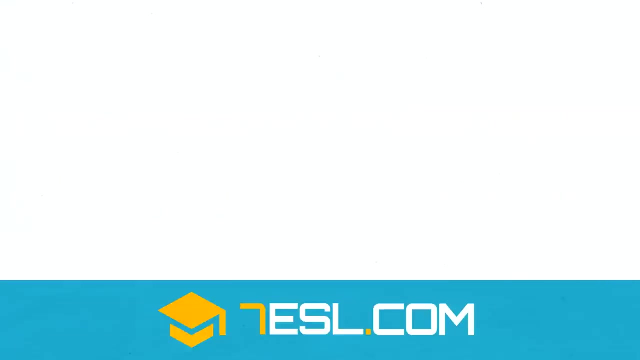 Exists: Percent 미나: 2, 6, 7, 8, 9, 10, 11, 11, 14, 15, 16, 16, 17, 18, 19, 20, 23, 23, 24, 25, 26, 27, 30. 28. 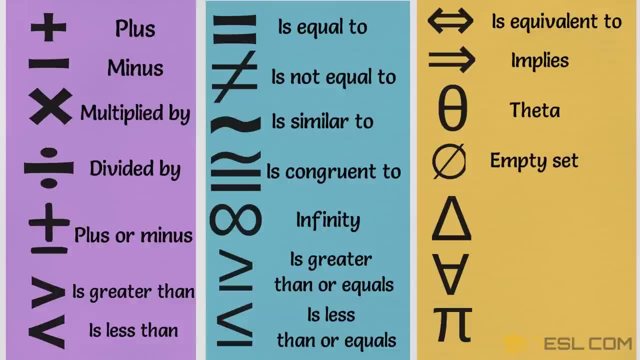 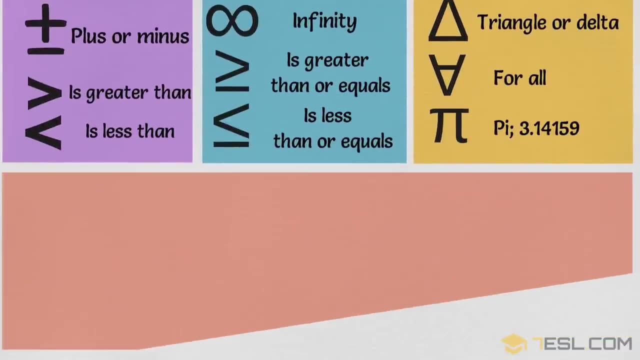 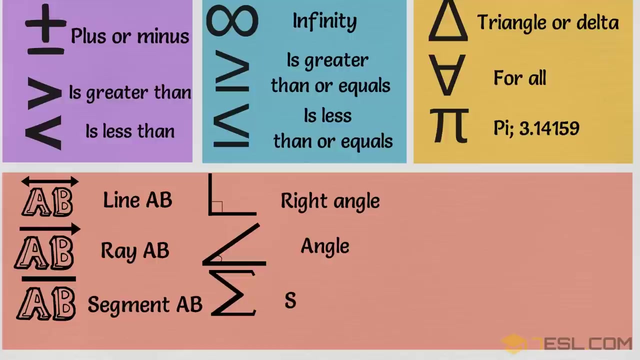 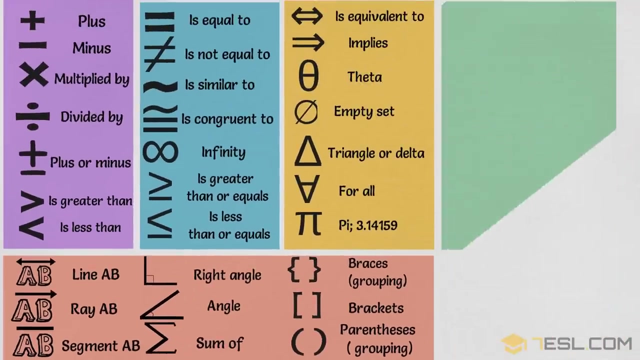 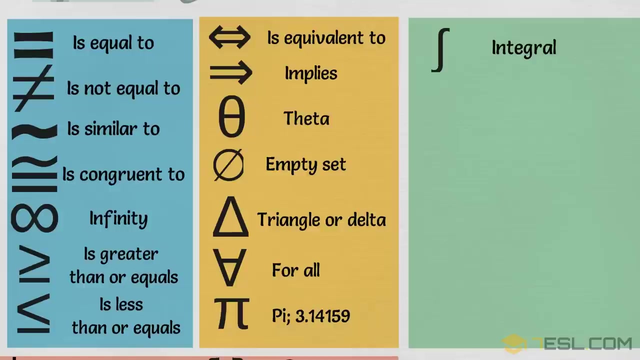 Empty set. Triangle or delta For all. Pi 3.14159 olé. LINE A-B. LINE A-B, Front angle, angle. sum of braces, grouping brackets, parentheses grouping. integral intersection of two sets. union of two sets. 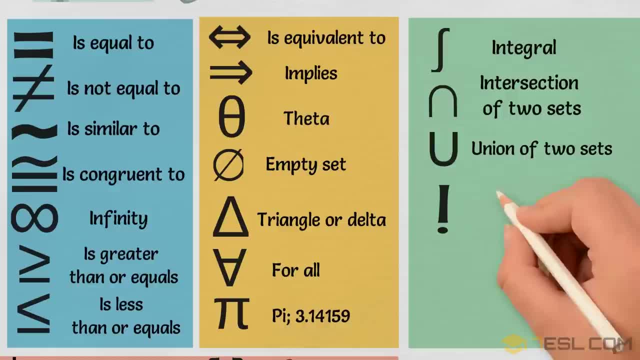 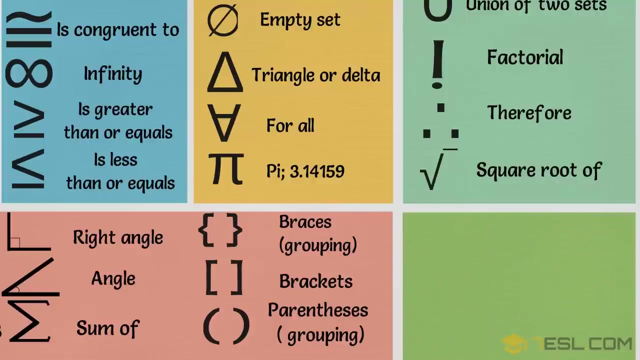 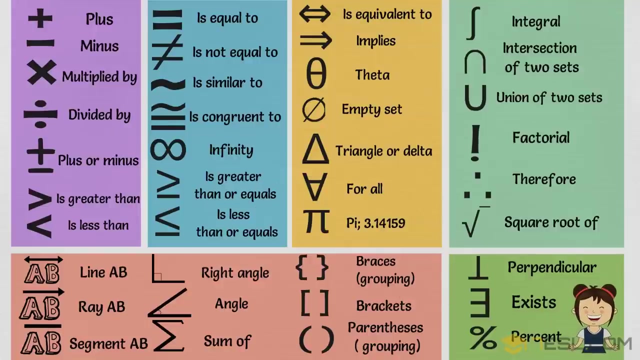 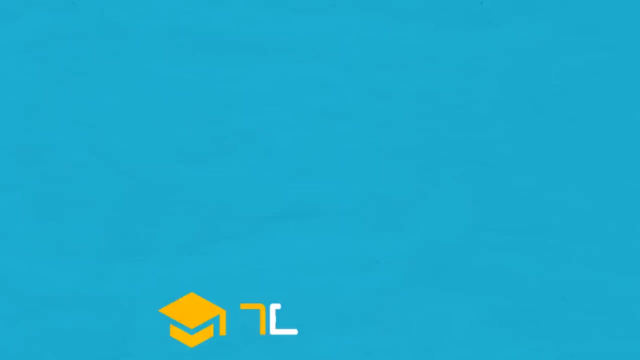 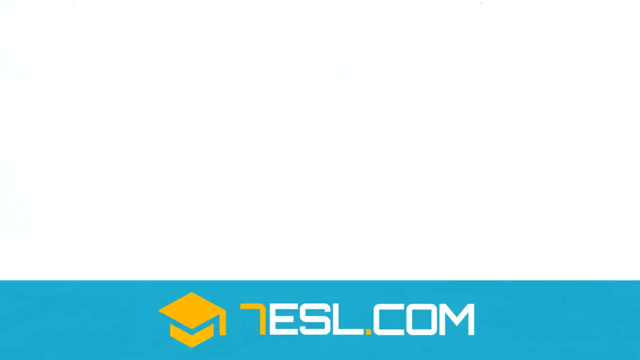